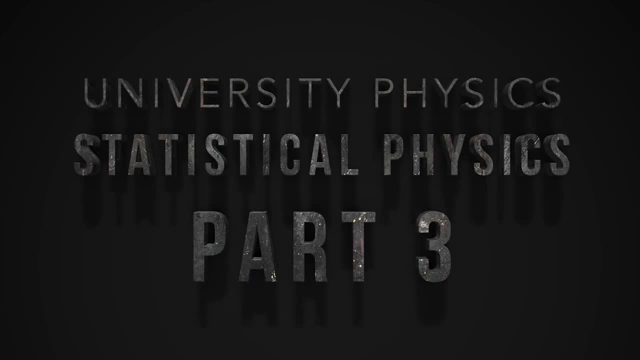 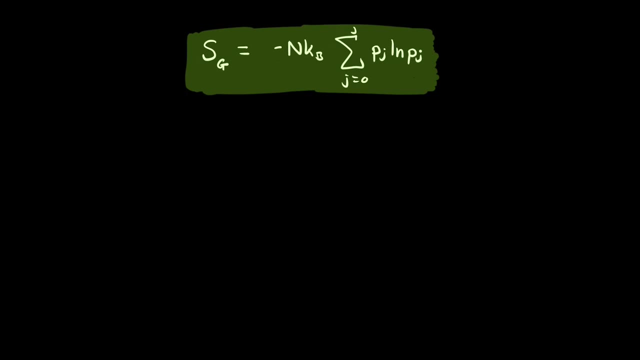 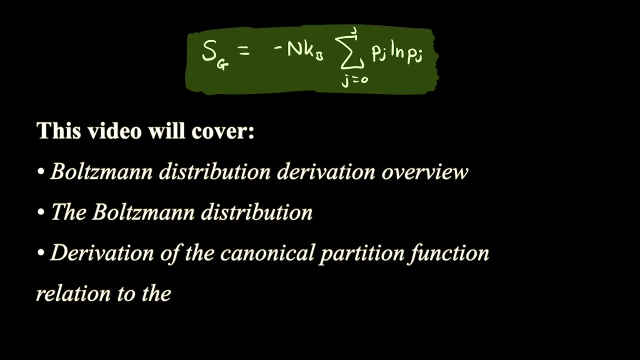 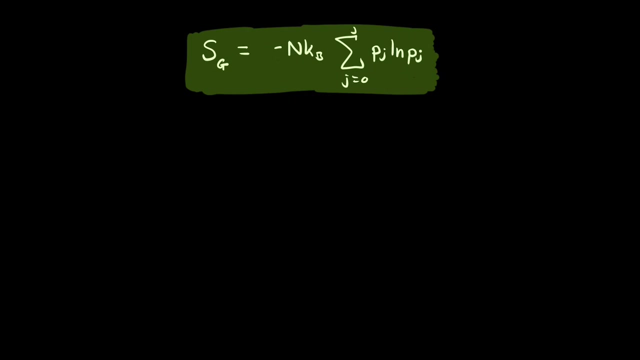 Hey guys and welcome to my next video in my series of videos on statistical mechanics. In the last episode I derived this which is called the Gibbs canonical entropy, and it's a statistical definition of entropy that we derived from the Boltzmann distribution, and in deriving it we basically had 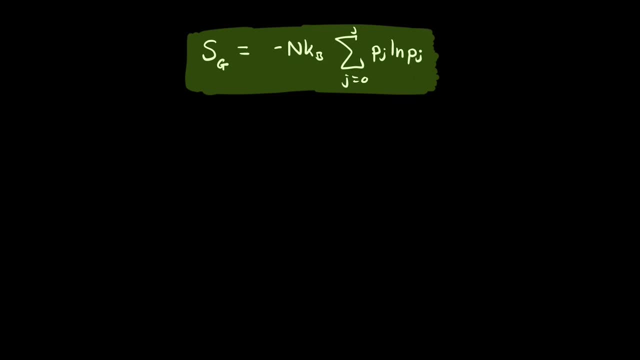 to make the assumption that the total number of microstates omega is approximately equal to the number of microstates in the most probable macrostate, w. so w max was. so we kind of had to make this approximation, which at first glance seemed a little bit weird, to approximate that. 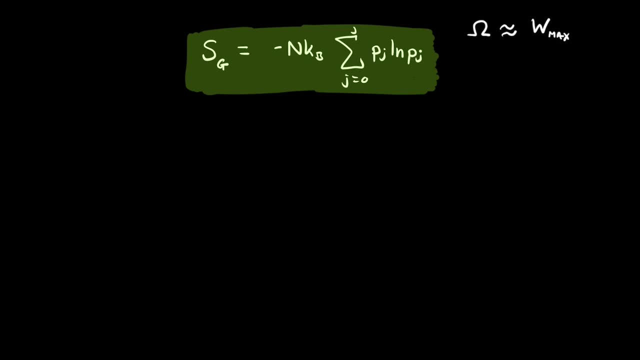 but we found that it is actually true for a sufficiently large number, and you'll find that it will be true, and you'll find that it is a valid approximation. We also had to use Stirling's formula, which said that the log of n factorial is approximately equal to n log n minus n. right here? so, yeah, we did use a couple of. 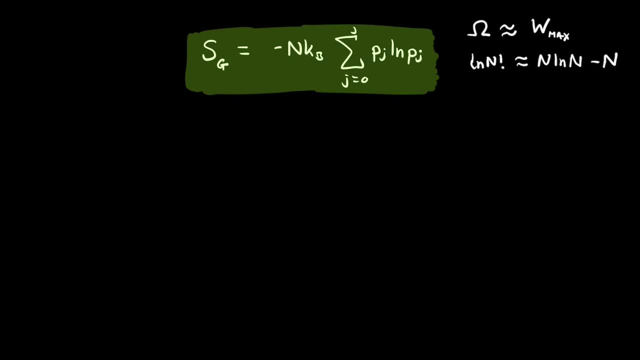 approximations along the way. you know, physics isn't perfect, I guess, but with a bit of mathematical, mathematical trickery, then we ended up with this result right here, which is the Gibbs entropy. Now, from this in this episode, I am going to sort of semi-derive kind of tell you. 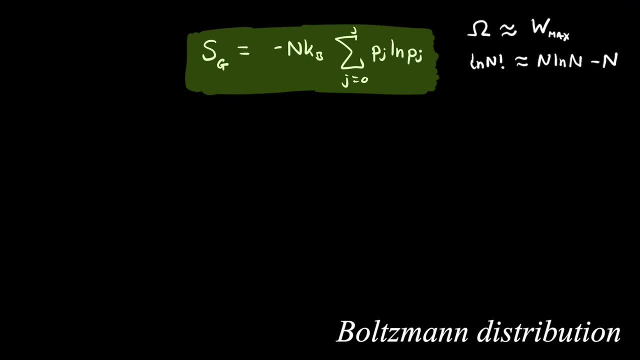 how you would derive what's called the Boltzmann distribution. I'm not actually going to go into the full details of the maths because you probably it's very advanced and you probably won't need to know it, particularly if you're studying university in your first or second year. you won't know how. 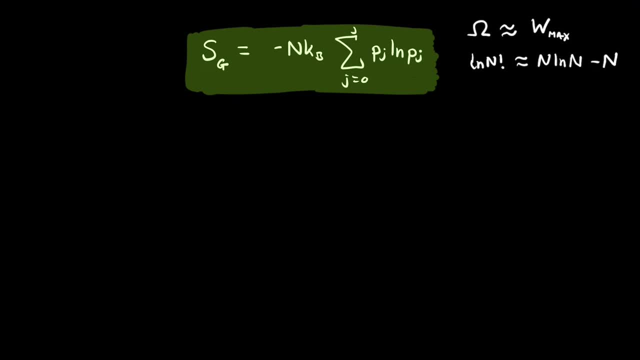 to derive this. but I'm basically just going to kind of go over it so that you kind of know how it is derived. but you probably will not have to do this derivation in your exam- at least I'm assuming. so you know not, unless you're doing a particularly complicated thing. so I should probably 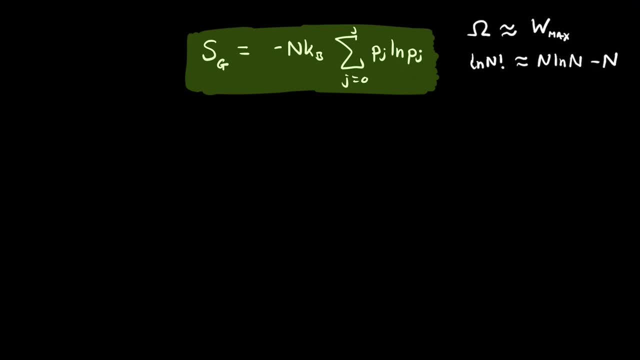 just mention what is the Boltzmann distribution. Well, the Boltzmann distribution is all about particles being in a certain energy level, so it's this probability of being so. p is the probability and e is the energy level. If we just sort of think intuitively about it, then we kind of figure. 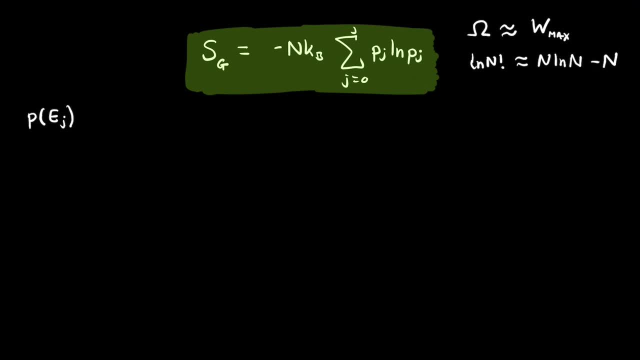 that particles tend to not really want to be in high energy levels. they'd kind of rather be in low energy levels, which is why I said before, you don't get frazzled when you, when you stare at the Sun. you don't get frazzled with x-rays and gamma rays, because there are more photons that are in. 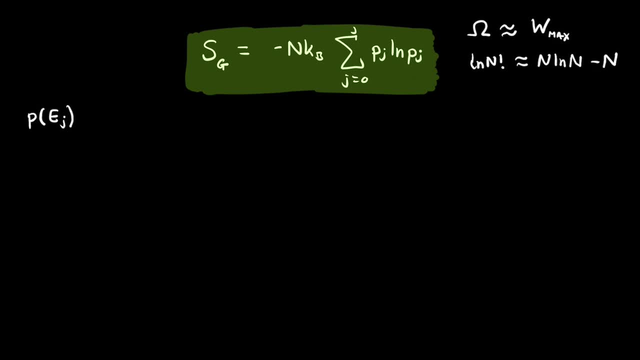 the sort of infrared and visible light range, range of the spectrum, rather than in the ultraviolet. so you know, nature tends to prefer lower energies and so you could probably expect the distribution, the Boltzmann distribution, which is all about distribution of energies, to look, you know. 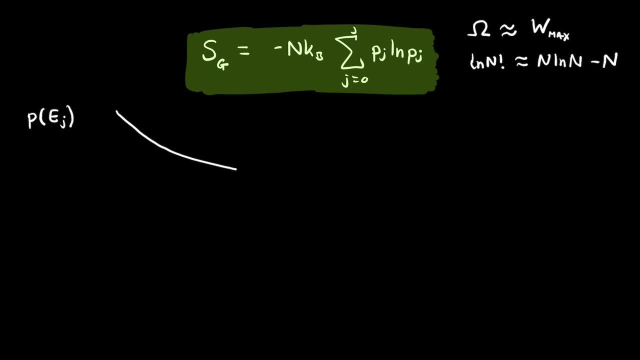 something like a sort of exponential tailing off things. so that's kind of the way it works. It's kind of going to be our guess. as it turns out it will turn out to be an exponentially tailing off graph. so Boltzmann is so intuitively we are right about that. but we're just going to sort of 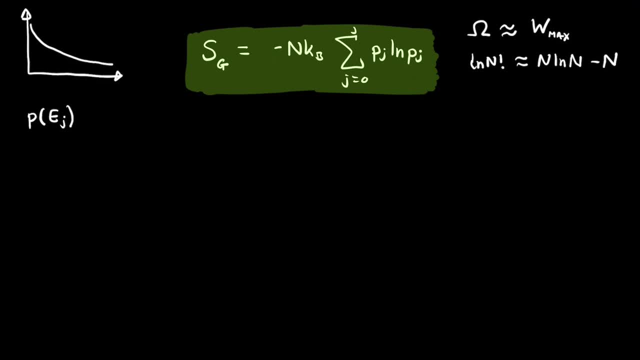 kind of derive. it just kind of show how it's derived. So the way in which we start to derive it is: we say that we want to maximize, we want to maximize the entropy sg, And in maximizing the entropy it kind of follows along from the second law of thermodynamics. we want 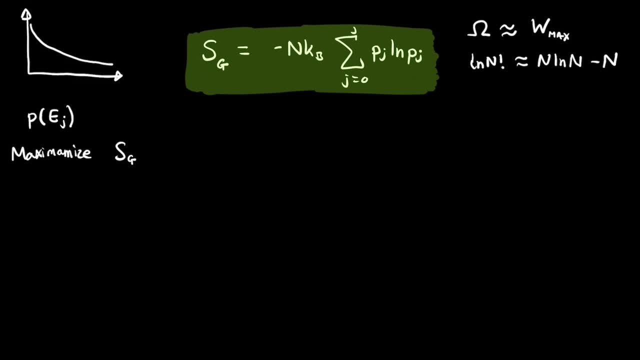 to find those macrostate probabilities that result in the highest entropy s right there. So that's basically what we're trying to do Now. the way in which we do it mathematically is using a method called Lagrange multipliers. Lagrange multipliers. 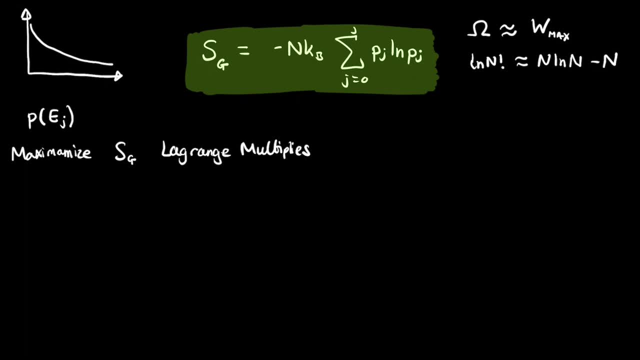 and And. basically, what this does is it's able to find local maxima and minima for a particular function. Now I've got to be honest, I don't really fully understand how it works. but I didn't have to, I didn't really have to understand how it works. All that you really need to know is basically how it's derived. 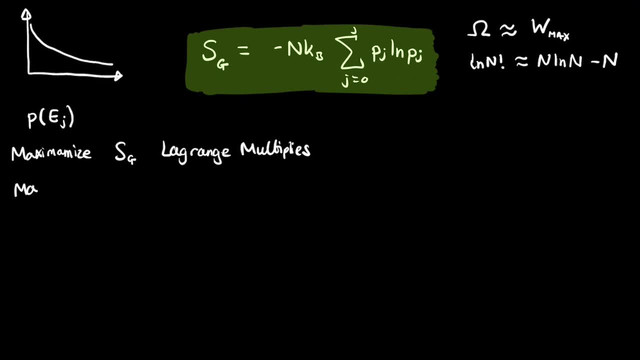 So the way in which you write this is that you want to maximize a function, f, And the way in which we write this is the function is of this variable pj. That's exactly the same as this right here, It's just I've not bothered writing out this bracket. 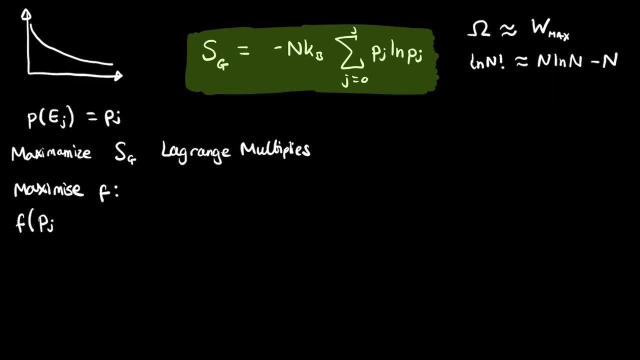 I should just put that's equal to pj. I want to maximize pj And we just put these little squiggly brackets right here, subject to a couple of constraint variables, And these are just called lambda and gamma for now. So we're trying to maximize this f, which is a function of these three variables subject to constraints, right here. 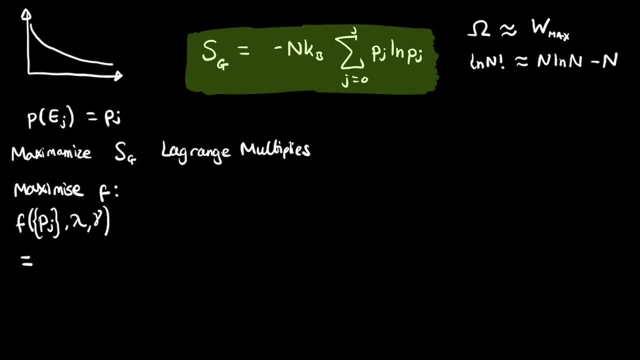 So f is our function. So what is our function that we want to maximize? Well, it's this right here, isn't it? It's our canonical Gibbs entropy. So we're going to rewrite this as sg, which is, of course, a function of the pj's. 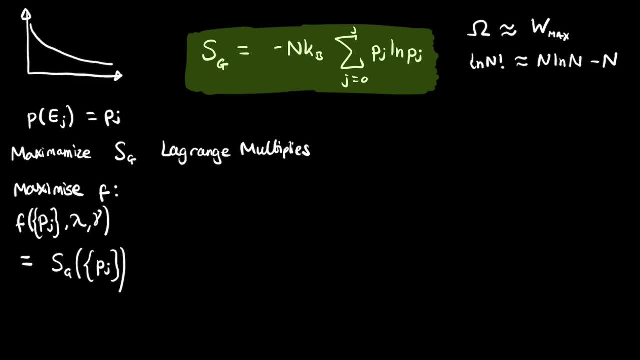 So this is our function that we're trying to maximize. We're trying to maximize the entropy. Now we want to add on to this our constraints. Now I did actually mention this a couple of videos ago. I didn't mention it in the last video, but we had a couple of definitions for n- the number of particles, and u- the average energy. 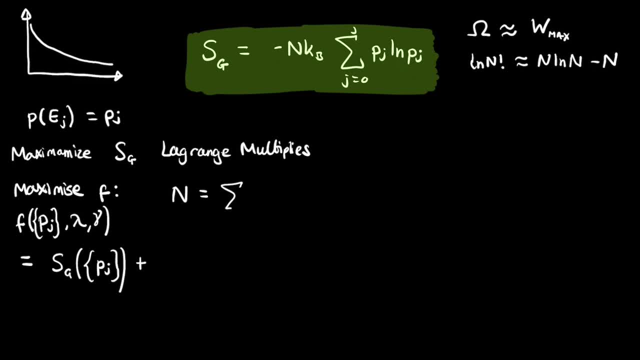 n, the total number of particles is equal to the sum from j equals zero- to j of nj. so summing over all the energy levels, counting the number of particles in each energy level, which is also equal to n, which I showed in the last video, 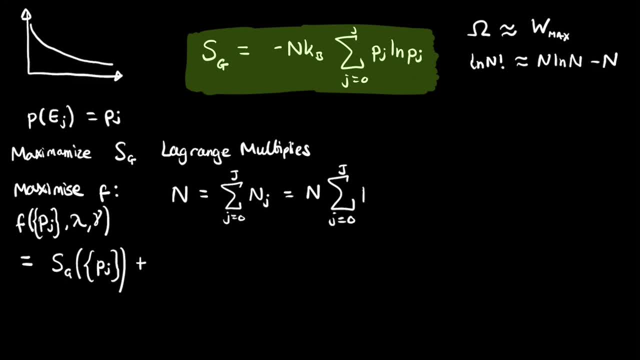 sum from j equals zero to capital J of pj, right here. So this is kind of, if you like, our normalization condition, such that you know the total number of particles is equal to the sum of all the probabilities And our other constraint is a. 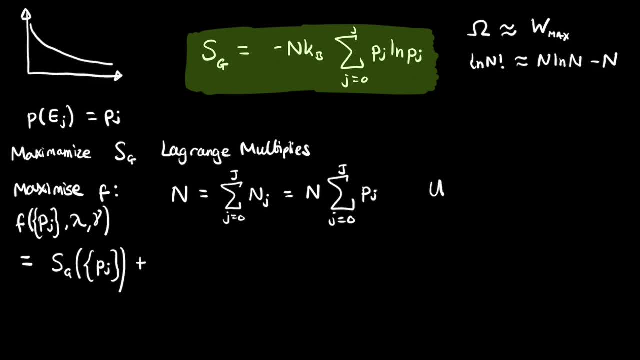 regarding the average energy, which is u And u. the average energy is equal to nj multiplied by the energy of the jth energy level, divided by the number of particles, And, of course, we're summing over j, And you could also rewrite this in terms of probability. 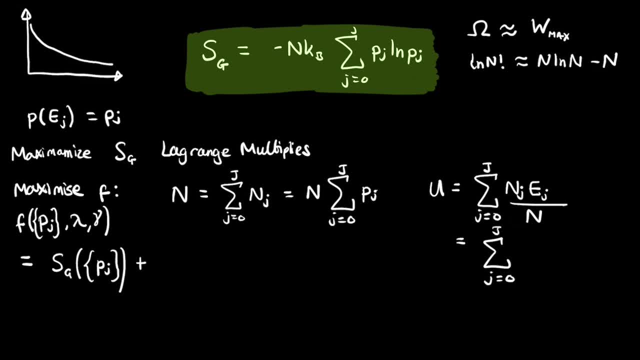 So u the average energy is from: j equals zero to j of pj, ej. So it's actually pretty much how you would work out the expectation value in any sort of statistical system. You probably did it in statistics, like in statistics at A-level. 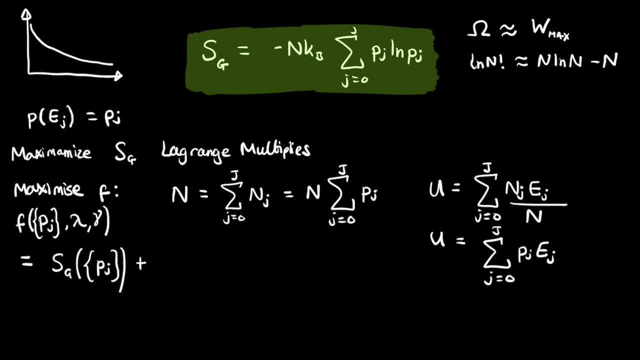 I certainly did anyway, And so you know it's how to, basically how you work out the average energy. So these are our two constraints, if you like. So we're now going to add these constraints on to the function that we're trying to maximize. 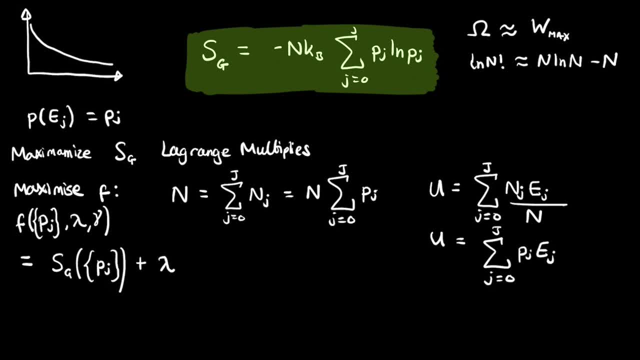 And the way we do this is we put this lambda term in front right here. We then write u minus n from the sum from j equals zero to j of ej multiplied by pj. right here. So we have average energy, fixed of course, and 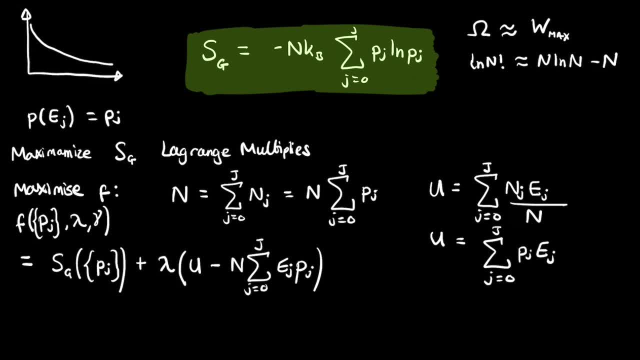 we want to try and make sure that this is a constraint right here. So we add on. So that's our first one. We then want to add on our second constraint, And that is that we want n this n right here to be exactly the same as this right here. 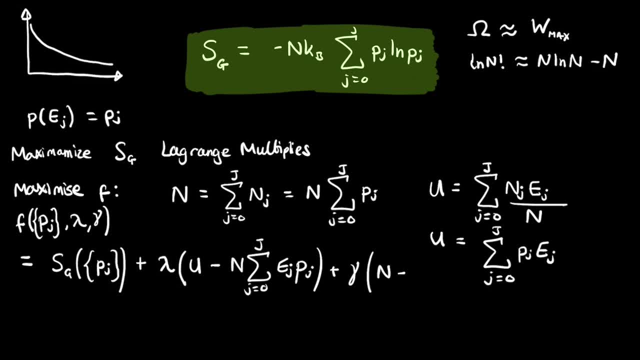 So these are our two constraints. These must happen. So we have n minus n summed from. we'll just move this out of the way because it's getting in the way. summed from, j equals zero to j of pj, right there. So these are our two constraints. 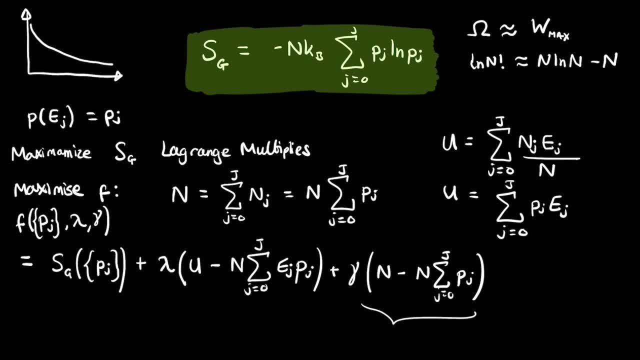 Here's our constraint regarding average energy And here's our normalization constraint, right here. And lambda and gamma are just constants that are given by, basically, the physics of the system. So our solution- which, again, I'm not really going to derive- 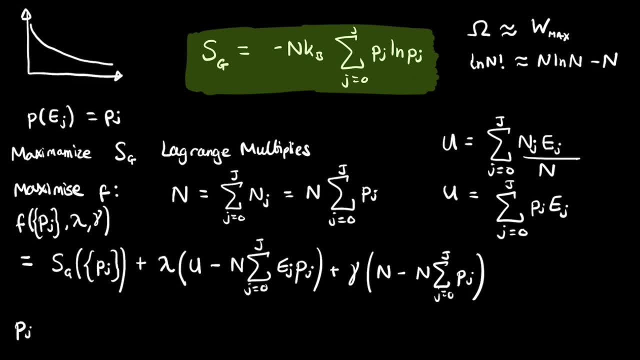 is that the probability is equal to some some normalization factor, just some constant to make sure it's equal to one multiplied by an exponential, which was kind of our initial guess up here. We kind of intuitively thought it was going to be exponential. 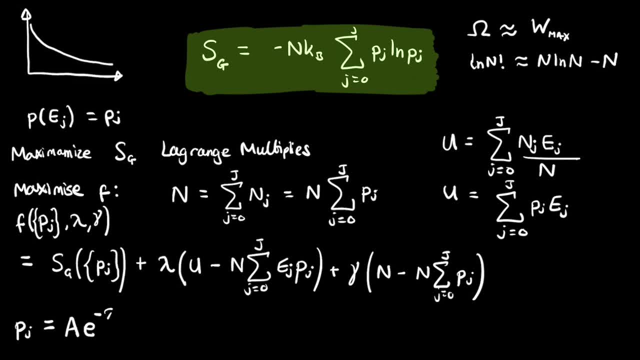 Multiplied by e or raised to the power of minus lambda ej. So this is basically the general form of the Boltzmann distribution. It's a dying exponential, It's an e to the minus curve, And so we use these two constraints. 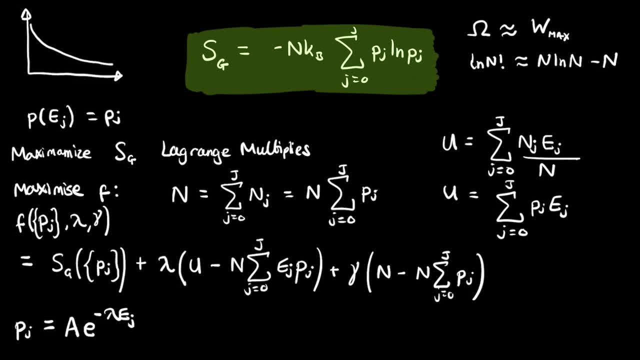 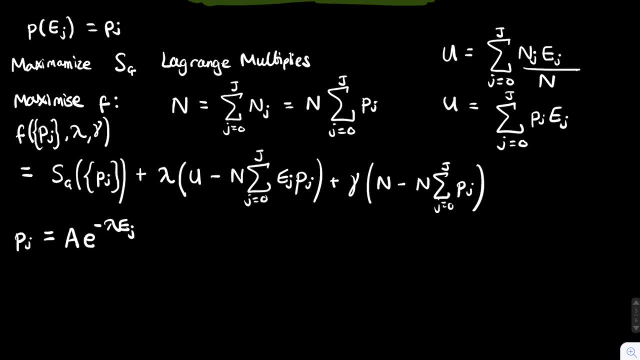 So we use these two constraints In the method of Lagrange multipliers to obtain this right here. Now I can finally reveal what this lambda is. As it happens, gamma doesn't appear in the final distribution, but lambda does, And lambda is actually equal to one over kbt. 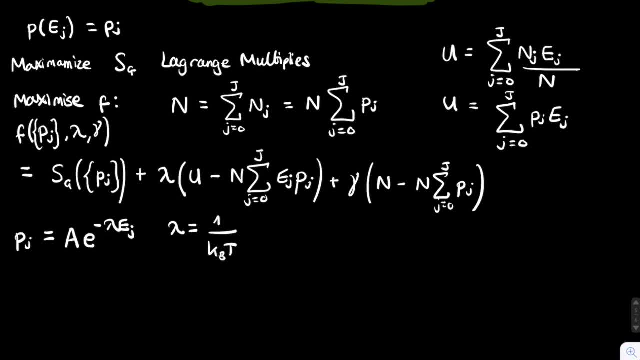 Now, of course, kbt is a measure of energy right here. So we simply multiply the temperature By the Boltzmann constant and we're going to get some sort of unit of energy. But we actually call it quite a lot in thermodynamics. 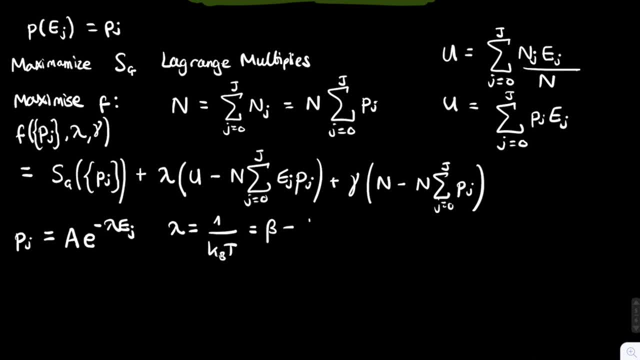 We call it beta and beta We kind of call the inverse temperature. It's called the inverse temperature. It's actually not a measure of temperature as such. It's actually a measure of one over energy that has the units of joules to the minus one. 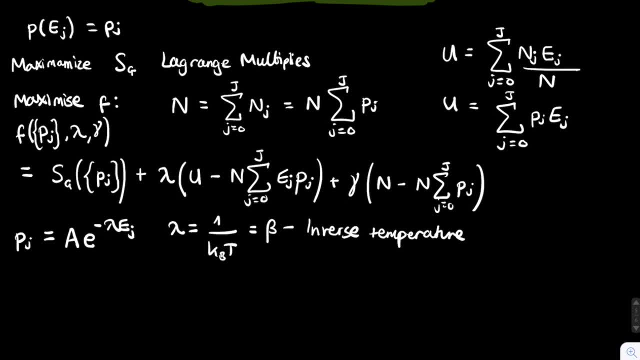 So basically it turns out that the higher the temperature is, the lower beta is, So when beta increases, the lower beta is, And when the temperature increases, then you basically get it much colder. So it's kind of a weird way of doing it, but it basically makes everything a lot easier to write. 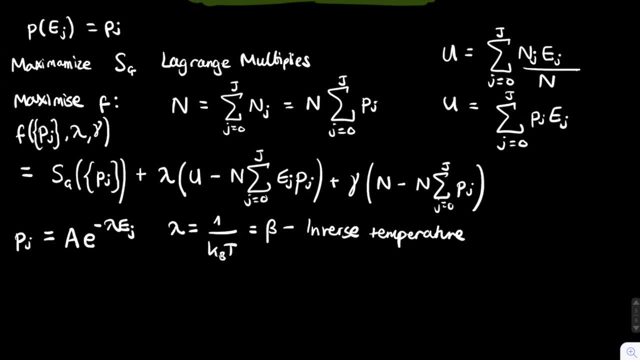 Because we find this one over kbt a hell of a lot in statistical mechanics, And so it's actually kind of just easier to just write this constant beta rather than having to keep on writing one over kbt all the time, And so we can use that. 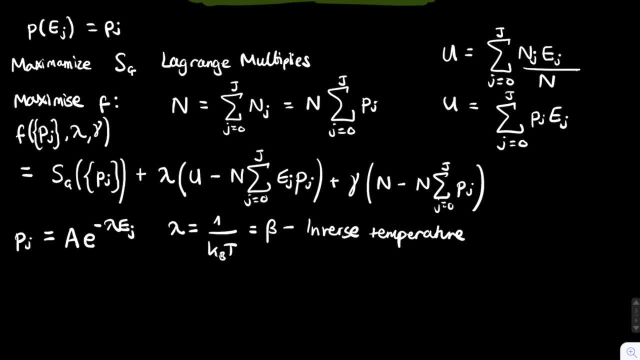 And so we can use that, And so we can use that, And so we can use this result to work out what lambda is. So, substituting this in, we get that pj is some normalization constant: a multiplied by e to the minus beta, ej. right here, 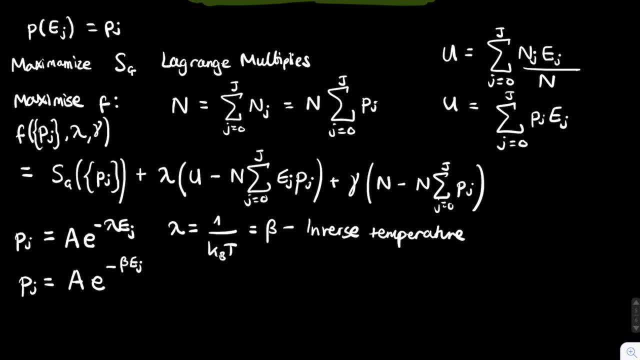 So now what we've got to do is work out what this normalization constant a is, And that's pretty easy. actually, We said that the sum from j equals zero to j Of all the probabilities pj from. also, if we sum over every single energy state, the sum of all the probabilities must equal one. 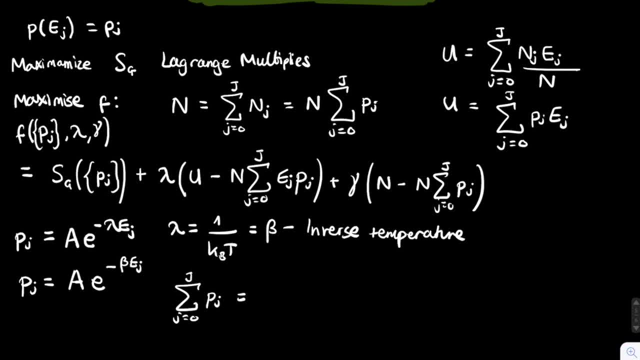 Again, I've said that quite a few times. You guys are probably sick to death of me hearing about that, But it is pretty damn important. So yeah, don't forget that. And that is equal to one. But what is pj right here? 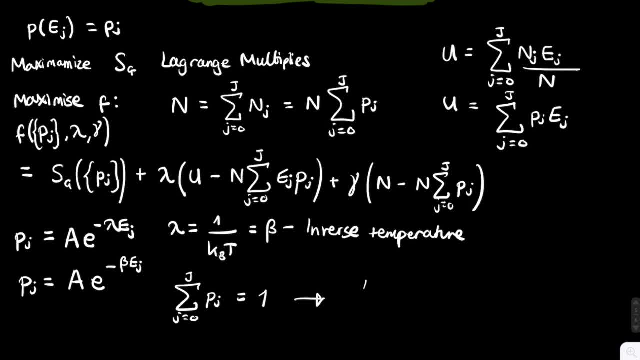 Well, we can simply substitute in what pj is into this equation Right here. So we go from the sum from j equals zero, to capital J of a, e to the minus beta, ej equals one. So I've just summed in what pj is right here. 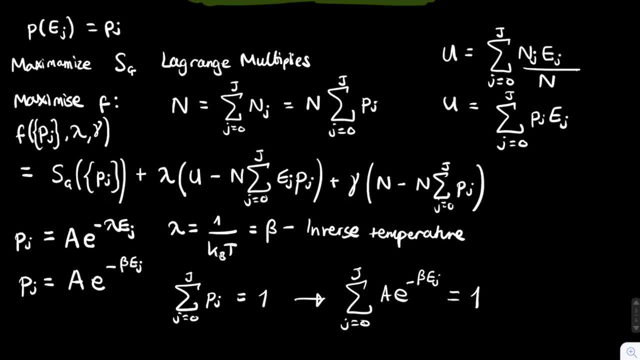 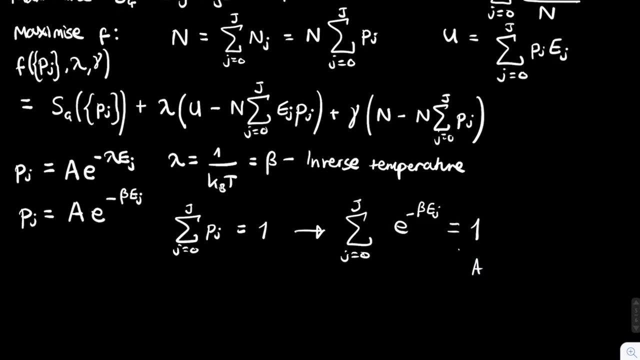 And so we can then take out this a out of the front of the sum Right there, And what I'm now going to do is divide both sides by a, So I get That one over a is simply equal to this sum right here. 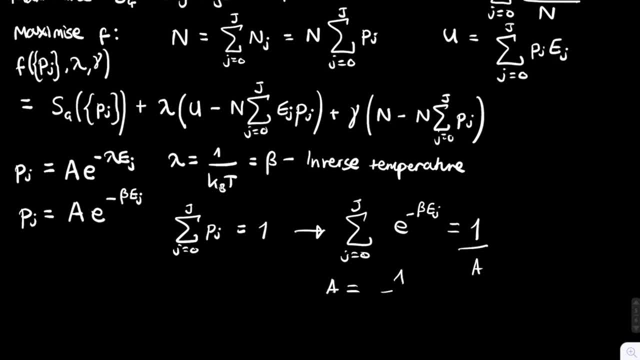 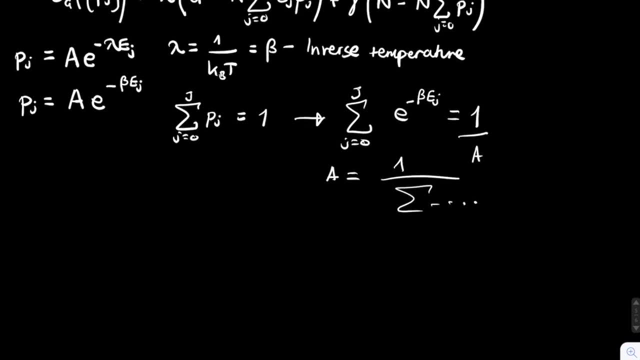 So a is therefore just equal to one over this sum. right here I'm not going to bother writing it all out, But you guys know what I mean. So we can now write our probability of it being in the jth energy level as e to the minus beta ej. 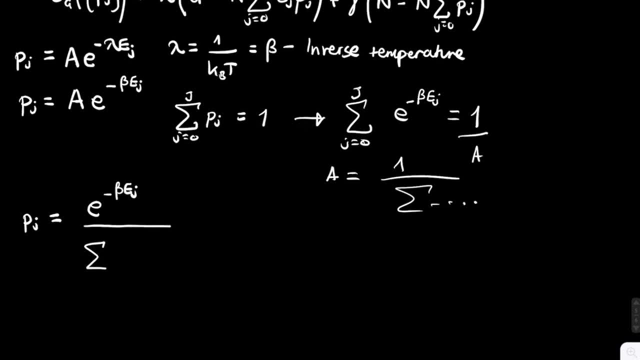 Divided by the sum From j equals zero to j, of e to the minus beta ej. and this is it, guys. this is the Boltzmann probability distribution, and it is very, very, very, very, very, very, very important. 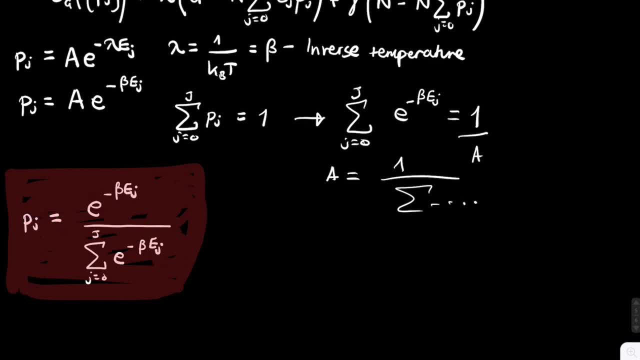 So I will not emphasize that enough. It's an incredibly important probability distribution formula And it basically is What we're going to be using a hell of a lot from here to come. so I'll just say it again: It's this term. right here is the probability of it being in the jth energy level. beta is the inverse temperature. 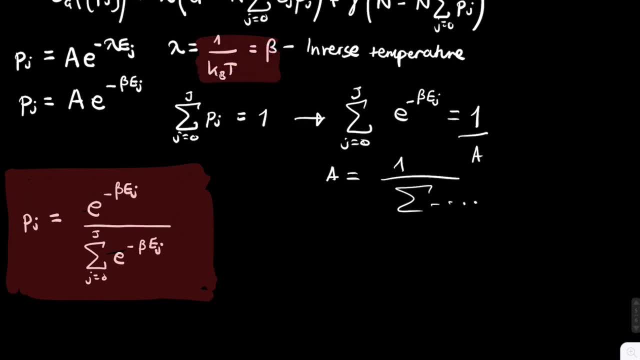 I'll just highlight that as well. The one over kbt is beta. right here It's just kind of a more convenient way of of writing temperature. So beta is just basically a measure of temperature. The higher beta is the lower temperature. I know it's a bit weird, but they get an. ej is the jth energy level. 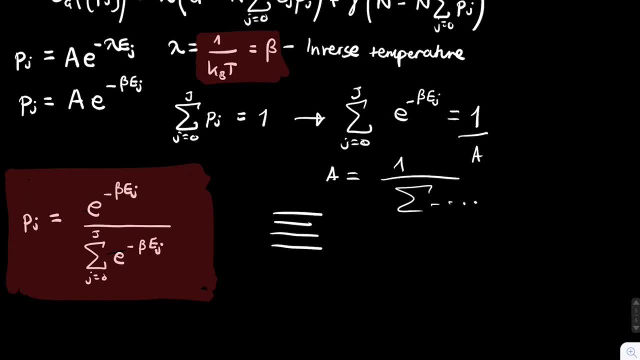 So remember our set of energy levels. right here, This is maybe e1.. This is e2.. This is e3, right the way up to some random one. ej and j is just a summation dummy index right here. So there we go. 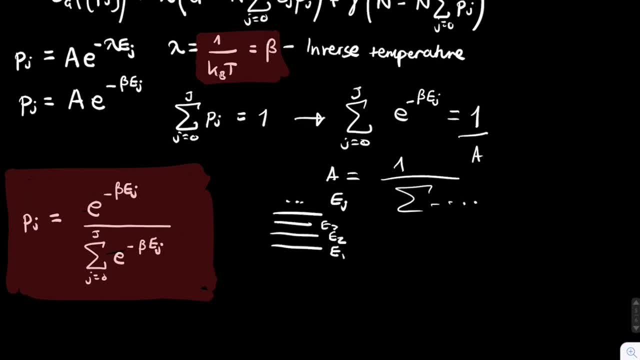 This is our probability distribution formula and it's very important. So there we go. This is our probability distribution formula and it's very important. You will have to know it pretty, pretty, pretty well. I would say I'm just going to make one small change and you guys are probably going to not like me for saying this. 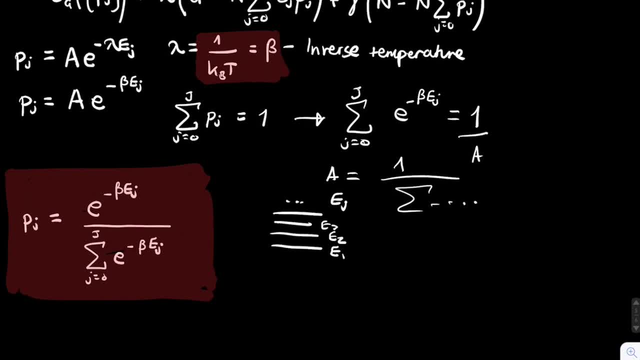 but we have kind of glossed over a fact. What if we have two difference states at the same energy? And the way I can draw this out visually is I'm going to draw my set of energy levels, but let's say this energy level right here. 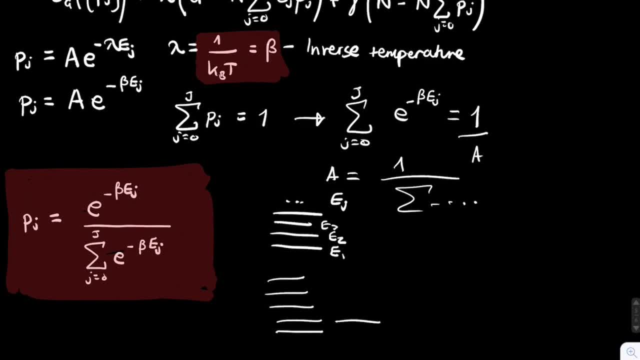 another state right there which is, you know, equally as probable. it's an equally probable microstate, and so, therefore, but it could also have this energy right here. so this is going to affect things, isn't it? and so what I'm actually going to do is I'm actually going to slightly change this formula. J is, of course, the 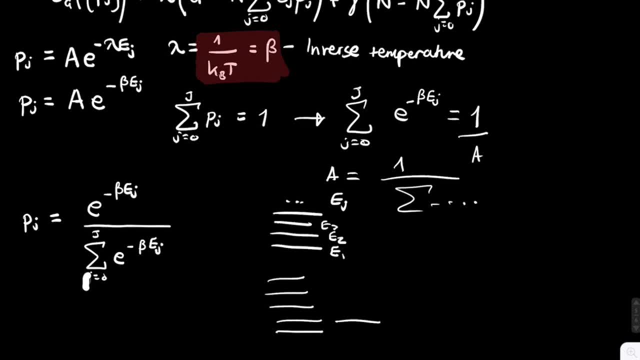 energy level. but I'm actually gonna, instead of use J, I'm just going to use K right here. so we're going to go from K equals zero to J capital, J still the same, and we're just going to change this out for K right here. and so the reason: 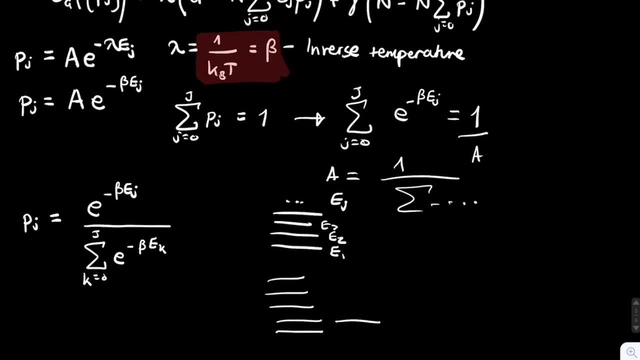 I've done. this is that we could be- we're actually going to be- summing over energy levels rather than summing over states. so, yeah, K is basically summing over all the different states, J is basically summing over all the different energy levels, and so you could have different states at the same energy level, for 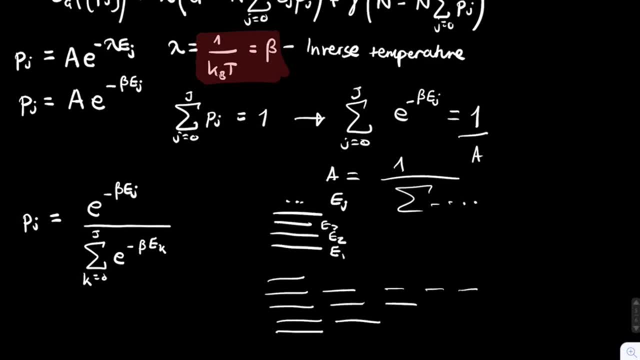 example, this one could have three, the this one could maybe have five or something, and you'll actually find this a lot, and we call this concept of the same energy with different states. we call it degeneracy, call it degeneracy and it's quite an important concept when 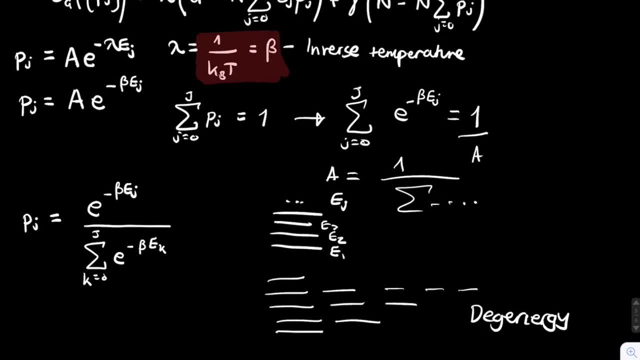 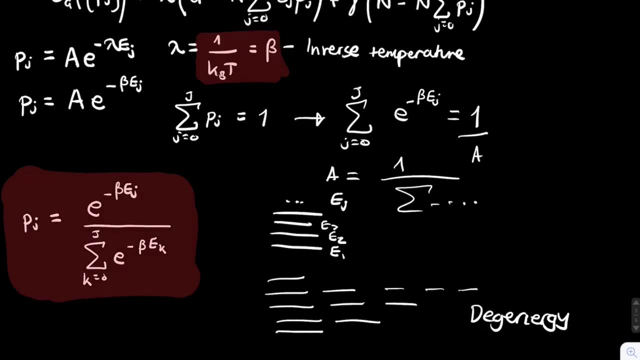 it comes to statistical physics, it's basically the same energy with different states right here. so there we go. so that is our slight modification. I'll, in fact, we rehighlight this. so it's essentially the same formula, it's just I've basically changed what I've called what I'm summing over. so instead of 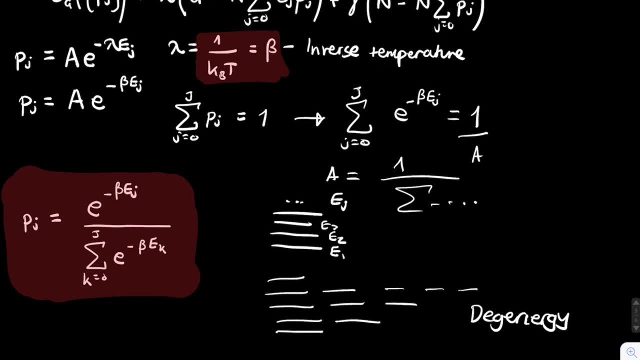 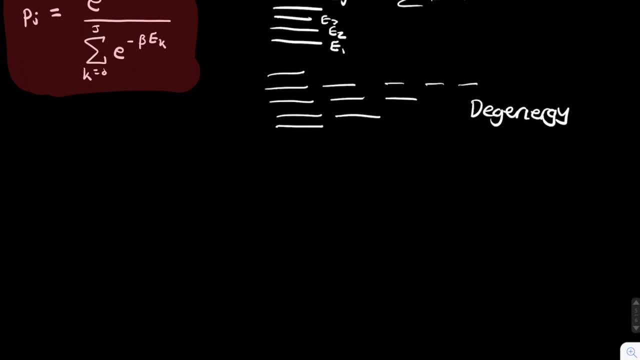 something over NG levels. I'm summing over all the different states. so there we go. here is our Boltzmann distribution. so now, what am I gonna do? well, I'm gonna do what I normally do with a new function: I'm gonna go ahead and graph this thing right here. so let's go ahead and graph. 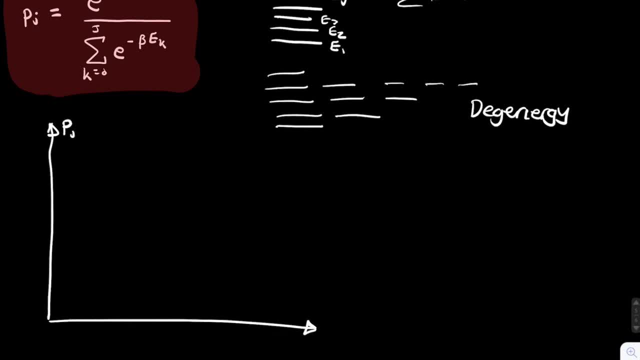 half the probability of it being in the jth energy level against the energy level right here. of course, you know we've got probability, which is the function, and, and it's a function of energy. so what are we going to get? well, remember, we're talking about discrete energy levels right here. 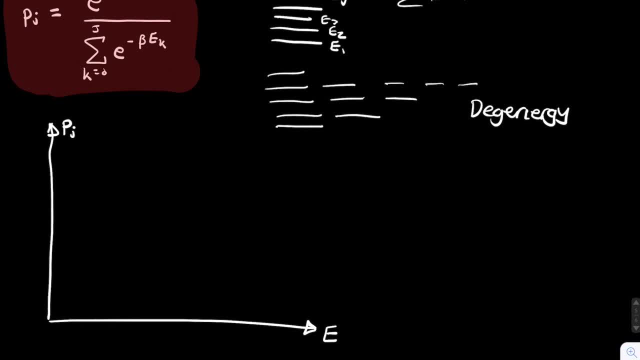 so we're going to get that instead of like a smooth, continuous graph. we're going to get some dots, but we're going to just essentially join them up. join the dots and we will see that it is an exponential graph. so what happens when the energy is zero? well, if the energy is zero, 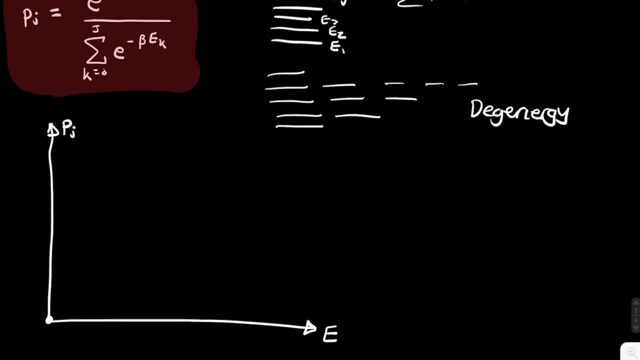 then this term, this whole term right here, this whole term within the exponential, is going to be zero as well, and we know that e to the power of zero is just simply one. If you raise anything to the 0th power, then you will get 1, and E is no exception. 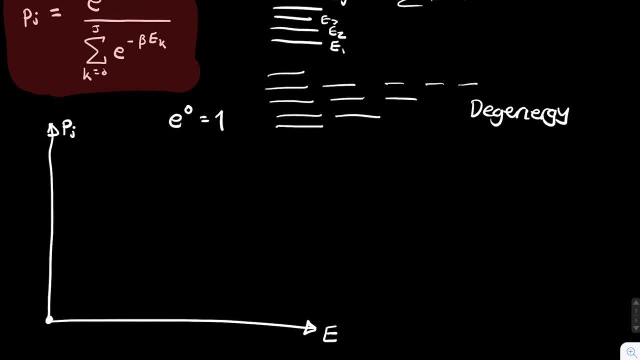 So, therefore, when E is 0, you are just going to end up with this right here, this 1 over this summation term. right here, Now, I'm going to call this term in the denominator. right here, I'm going to give it a name. 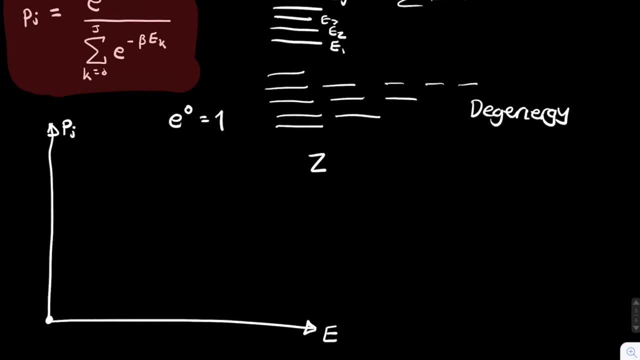 I'm going to call it Z. I know I used A earlier, but I'm going to call it Z right now And I'm not going to tell you what Z is right yet, but I'm just going to call Z. the sum over states from K equals 0 to J, of E to the minus beta E, K. 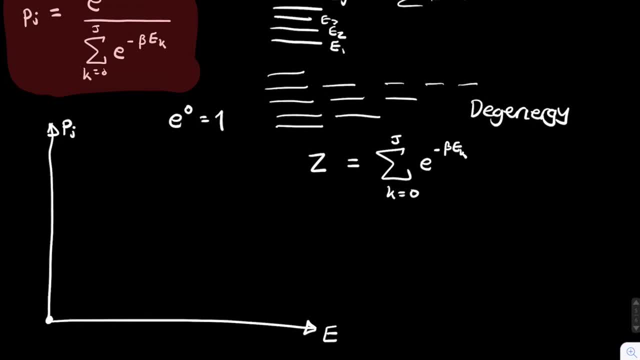 Remember, don't worry about the K, it's just simply another dummy summation index right here, And I'm going to just call it Z. So what's this graph going to look like? Well, it's going to hit this axis here. so that term, remember, is just 1.. 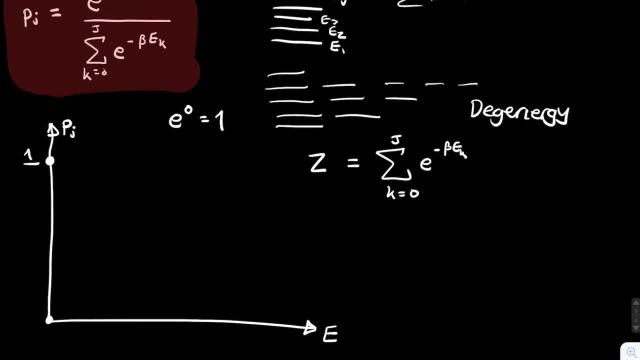 This term is just Z, so it's going to just simply be 1 over Z right here. And so what's going to happen? Well, we can see it's an exponential curve, but of course we're still dealing with discrete energy levels, right here. 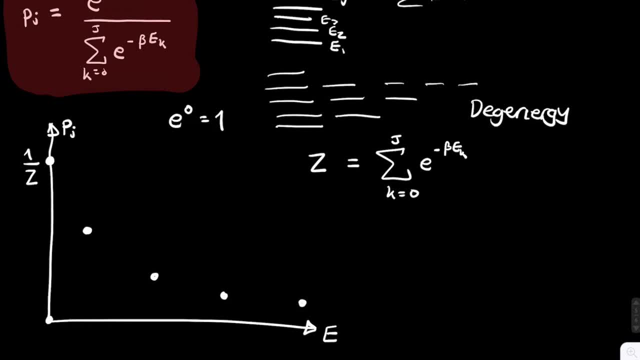 So we're just going to essentially draw out the dots and we find exactly what we thought we were going to find is that there was an exponential decrease. So I'm going to draw, I'm going to basically draw in the missing line. 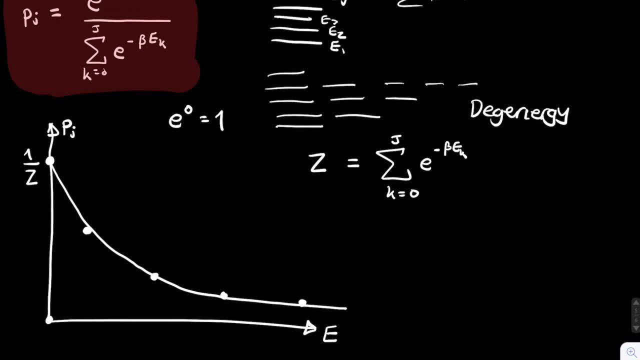 We're going to pretend It's continuous for a second. It's an exponential dying number. So basically, the higher the energy level, the less likely it is for a given temperature. Remember this: probability distribution is also a function of temperature. 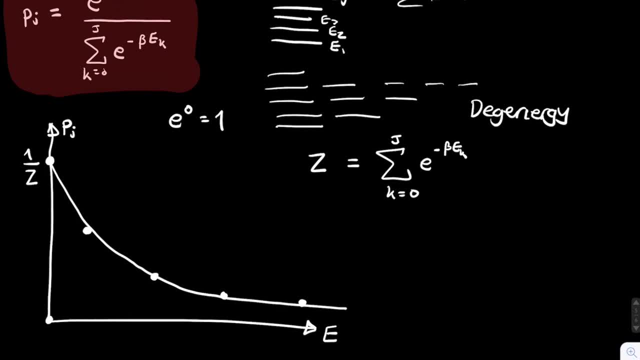 This is essentially what beta measures. And so what's going to happen to this distribution if we change the temperature? So if we lower the temperature, say, let's say we're going to lower the temperature, Well, this term isn't, It's going to change on the top right here. 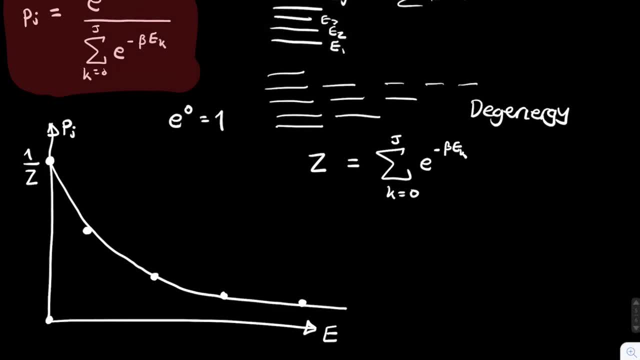 This term is still going to be 1, because that EJ will basically kill the whole thing. But what about this? right here? What's going to happen to this denominator? What's going to happen to Z? If the temperature decreases, then beta is going to increase, right here. 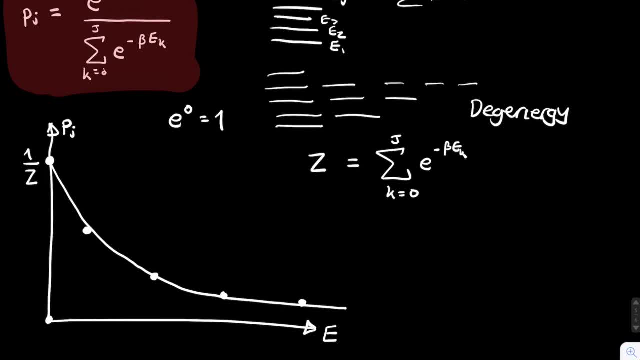 But what's going to happen? to an increasing negative, This whole exponential is going to decrease. So Therefore, if this whole exponential decreases, then all of the exponentials will decrease, So the sum of all the exponentials will decrease, And so we'll find that Z will decrease. 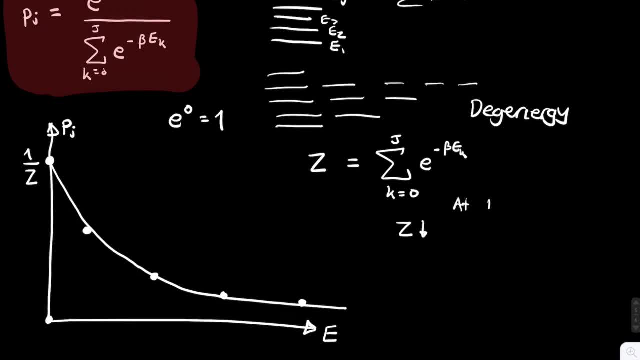 So at higher temperature, so at lower temperature, Z decreases. But what's going to happen to 1 over Z? Well, 1 over Z is actually going to increase. So you'll find that at lower temperature then you'll actually get a curve. that looks a bit more like this: 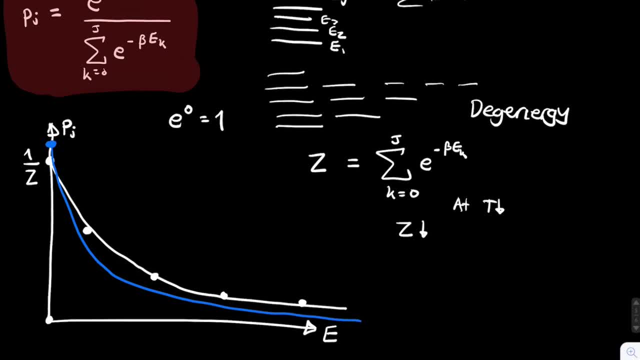 So it's the same exponential, but of course it's going to intercept the PJ axis at a higher point. So let's just call this Z prime. It's basically the new Z at the new temperature. So that is basically the temperature dependence of the Boltzmann distribution graph. 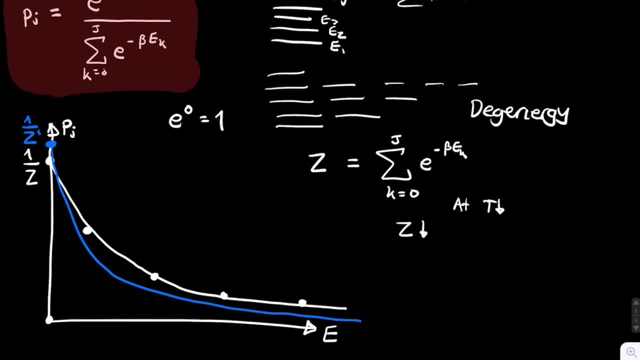 As you can see, increasing the temperature will make the graph a bit more sort of close to the corner, if you like, And I suppose in the limit you will get Basically a graph that looks essentially like that. This will be at very, very, very, very, very low temperature. 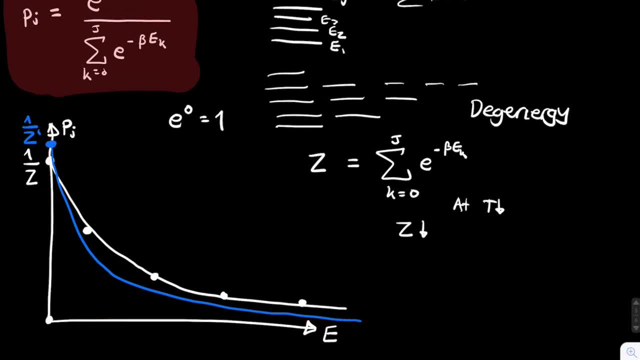 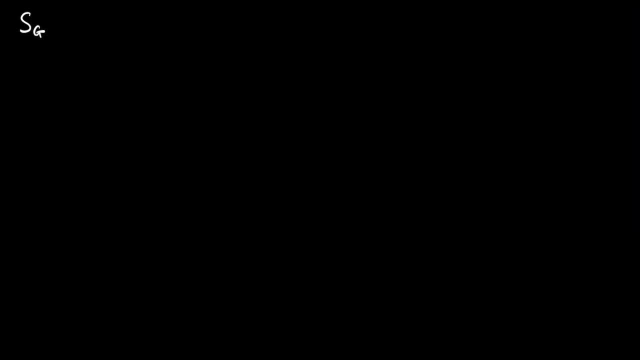 And, of course, absolute zero. you're going to get something a bit like that. It's just going to be a flat right angle. Now I'm going to go back to this formula for the entropy, the Gibbs formula for entropy SG. 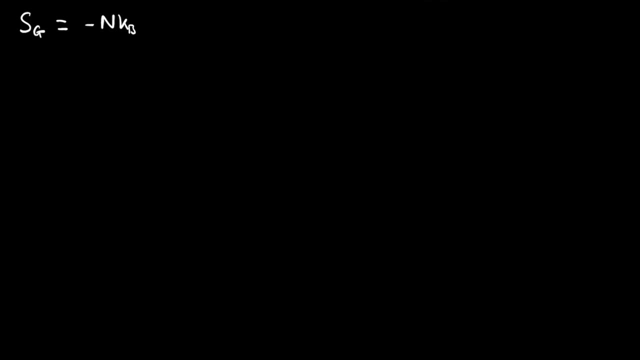 which was minus NKB, multiplied by the sum of PJ, log PJ. So this is our, This is our formula for the canonical Gibbs entropy, the entropy in the canonical ensemble, And so what I'm going to do is I'm now going to just simply take the entropy per particle. 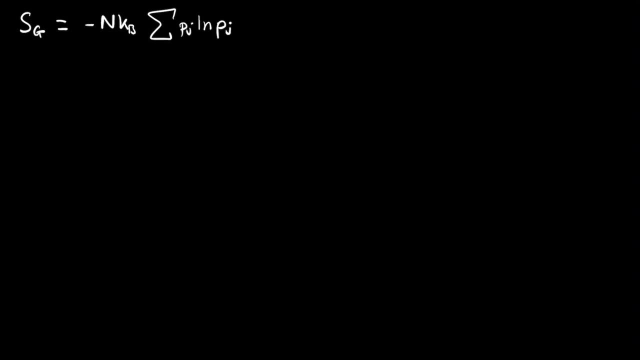 which basically means I'm just going to remove this N right here. So the entropy per particle- that's just simply going to be SG- equals minus KB times the sum. So the entropy of PJ log PJ- Oh whoops, PJ log PJ. 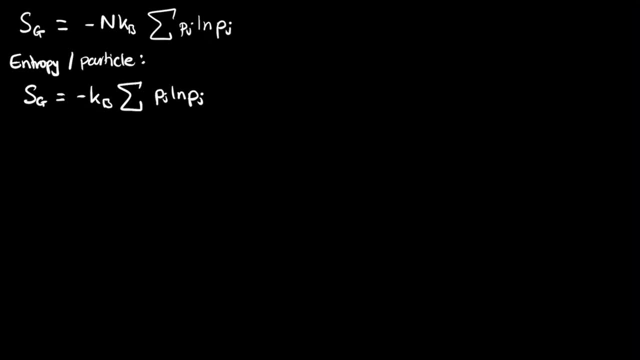 I'm not going to bother continuously writing in these summation indexes. We basically know that we're summing over all of the different energy levels. If it's J, then it's energy levels, If it's K, it's states, And I will come into what the difference between summing over energy levels and energy states are very shortly. 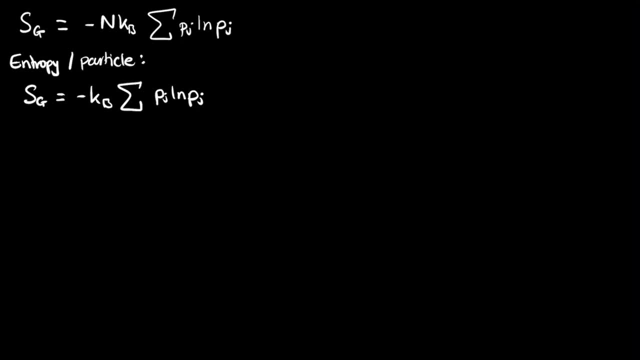 Very shortly, But for now we're just going to keep it simple. Everything is non-degenerate, Everything has one energy state per energy. So this is our entropy per particle. But what is this Pj right here? Well, we know what Pj is right- Pj we've just found from the Boltzmann distribution. 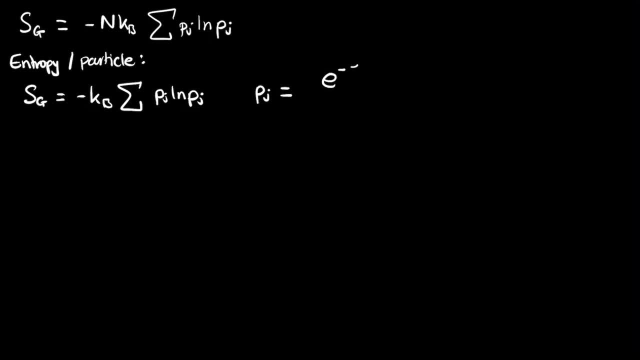 is e to the minus beta Ej divided by this Z right here. So this is what Pj is. So let's go ahead and substitute that into this entropy per particle right here, So we're going to have: Sg is minus Kb times the sum of Pj. Well, we can already take out this Z right here. So, because that's just a, 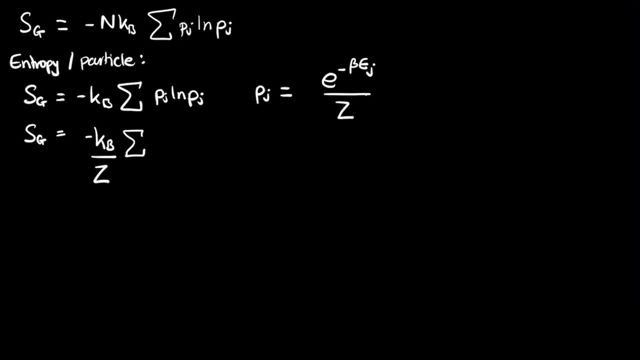 constant. that's not being summed over. So we're going to take out this Z right here, So that Z can immediately go out the front. e to the minus beta Ej times the log of e to the minus beta Ej divided by Z right here. So there we go. We've just basically substituted out Pj for Ej. 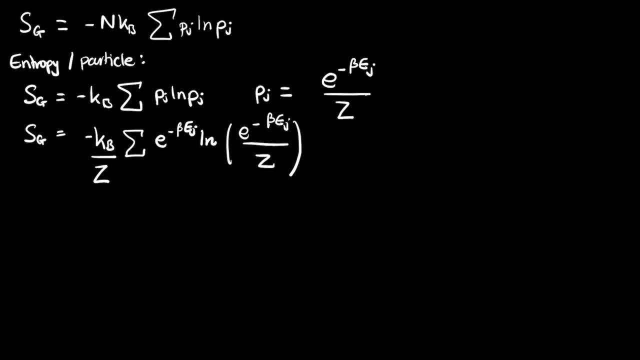 So we've written the entropy in terms of the energies. So let's go ahead and just tidy. Let's go ahead and just tidy. So let's go ahead and just tidy. Let's go ahead and just tidy. Let's go ahead and just tidy. 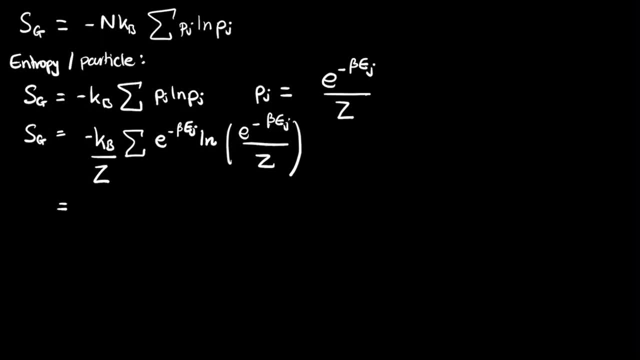 Let's go ahead and use our laws of logarithms in order to sort this term out right here, because it's a little bit messy at the moment. So we've got minus Kb divided by Z times the sum of e to the minus beta Ej, And we're now going to get two terms right here. We're going to get the. 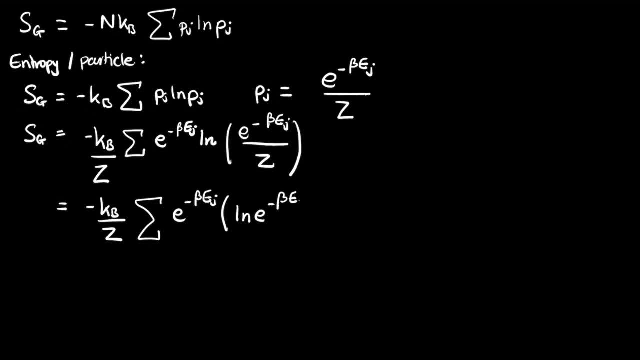 log of e to the minus beta Ej minus the log of Z. So there we go And, just as what happened before, this is going to now split into two different sums. So we've got minus Kb over Z. We're going to get the first sum, which is e to the minus beta Ej. 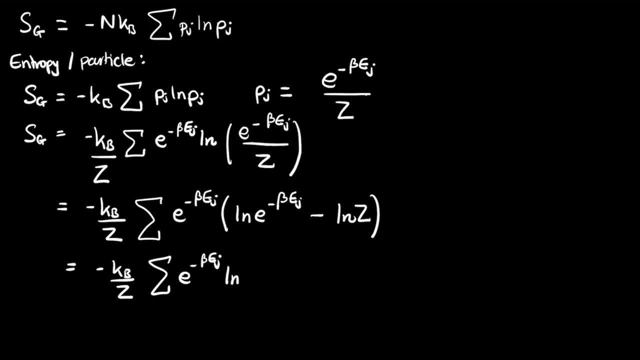 log of e to the minus beta Ej. That's our first sum. You can probably tell what's going to happen to this log and this E right here. But don't worry, I won't do it quite yet. Minus, let's put some brackets around this so we don't 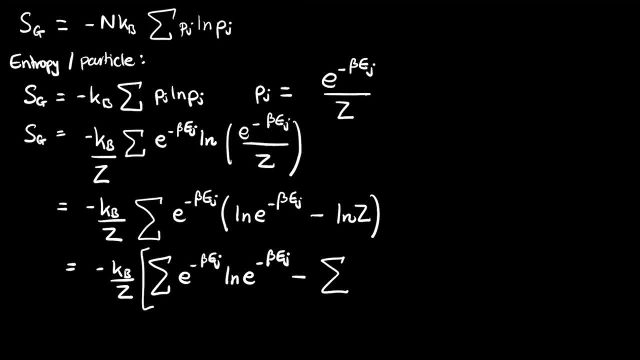 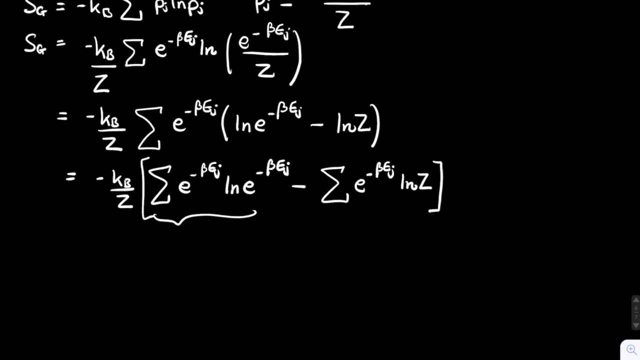 make a silly mistake. The sum over energies of e to the minus beta Ej times the log of Z, So this term is going to be fairly clear. what's going to happen to this? This is going to be simply Kb over Z, E to the minus beta Ej. 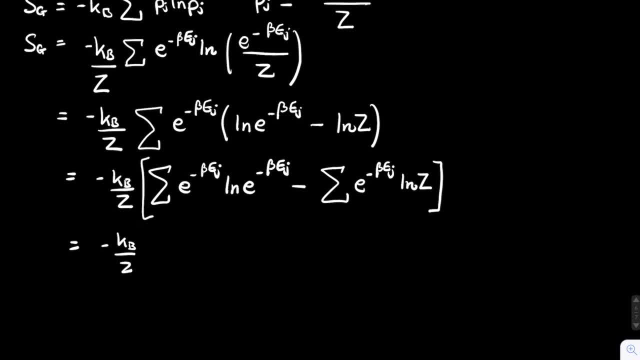 So log of e to the. anything is just going to be whatever's in here. So fairly obvious what happens to that. So we're going to get sum of minus beta Ej multiplied by e to the minus beta Ej And we're going to get minus. 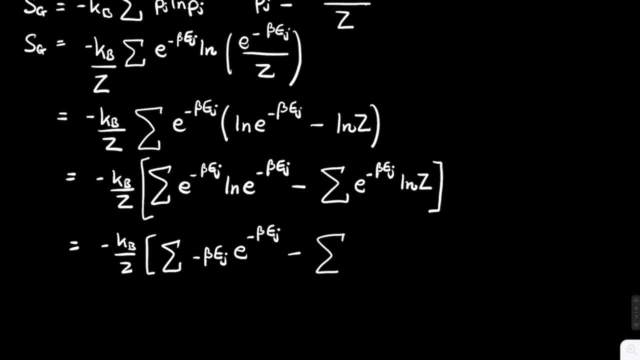 And this term right here is still going to be exactly the same E to the minus beta, Ej And the log Z. we can kind of put out the front right here. So here is our log of Z term, just coming out the front right here. 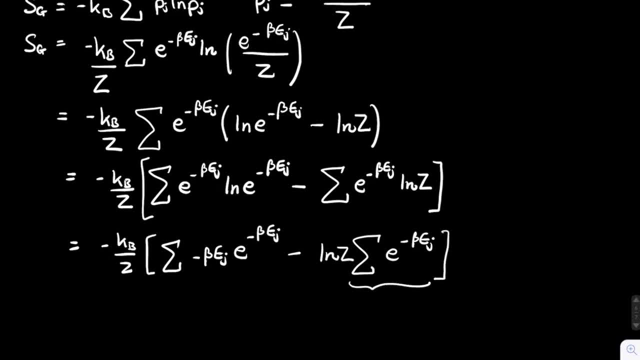 So there we go. But what is this term right here? This term right here is just well, some e to the minus beta Ej. That is exactly what we said was Z. Z is just simply equal to the sum over all the exponentials of all of the different energy levels. 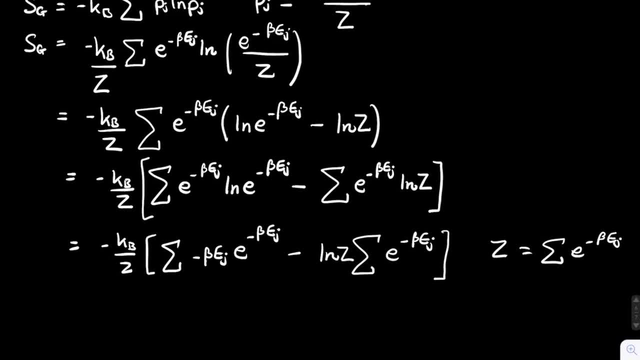 That is the definition of Z, So we can simply just replace the sum with Z. So we're going to get Z times the log of Z right there, So that condenses down quite nicely. And now we're going to go ahead and divide all of this. 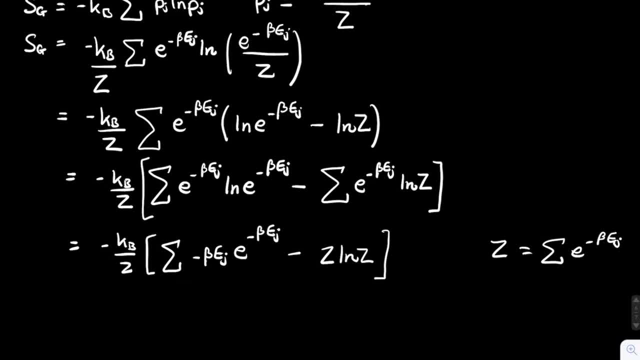 We're going to divide everything in here. We're going to divide it by Z And we're going to hence multiply this by Z. So we're going to get minus Kb, And instead of dividing by Z, we're just going to divide each of these terms by Z. 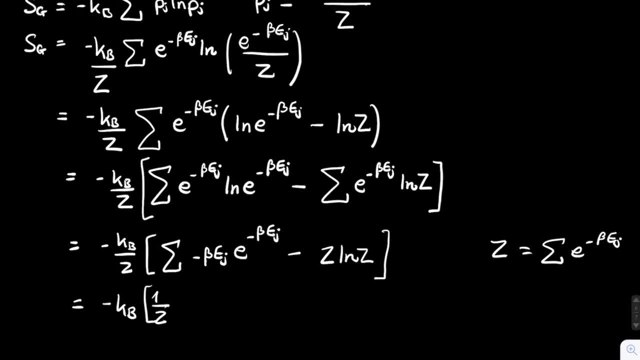 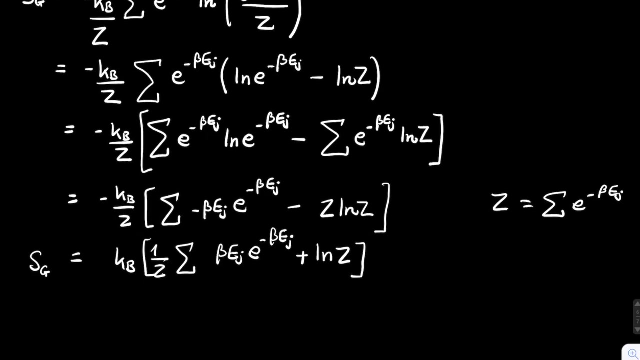 1 over Z. So multiply by the sum of minus beta Ej E to the minus beta Ej, Minus log Z Right here, And so that is the Gibbs entropy. So now, what are we going to do? Well, this beta can kind of just come out the front right here. 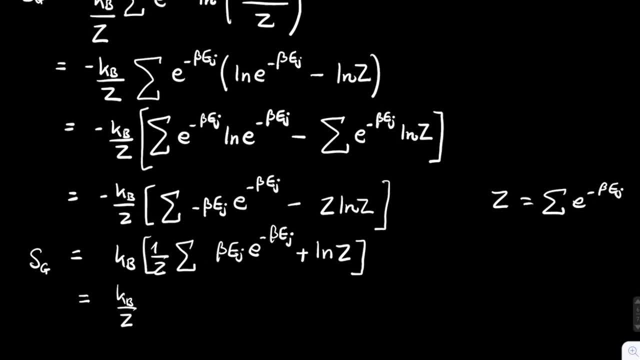 So let's just go ahead and rewrite Kb divided by Z times, beta times, the sum of Ej E to the minus beta Ej Plus. let's just go ahead and expand out this bracket again: Kb, Kb, Kb, Kb, Kb. 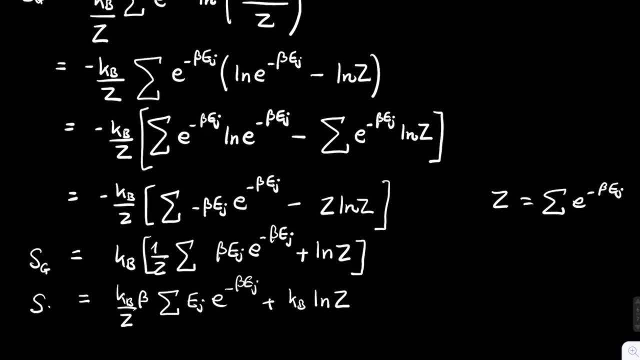 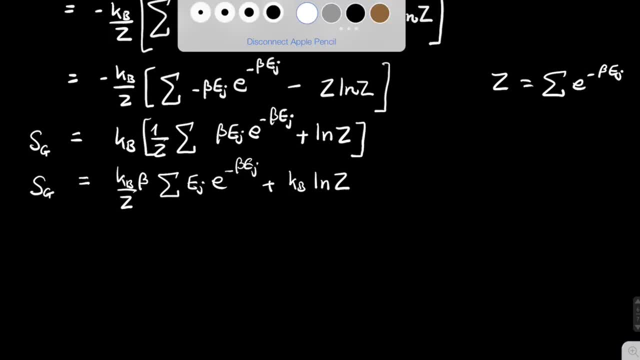 Log of Z Right here. So this is our Gibbs entropy. Now we can in fact, identify this term right here. Let me just highlight it: This term right here. What is this? We have some of our energies, E to the minus beta, Ej. 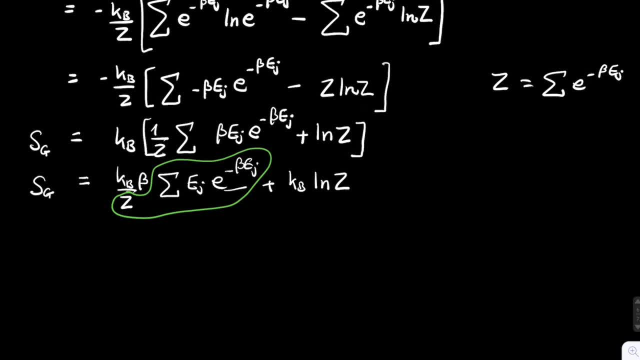 But what is this? E to the minus beta Ej divided by Z? Well, this is just Pj. Pj is equal to E to the minus beta Ej divided by Z. Right here This is our Boltzmann probability distribution formula, So therefore we can write that this is Kb times beta multiplied by the sum of Ej, Pj. 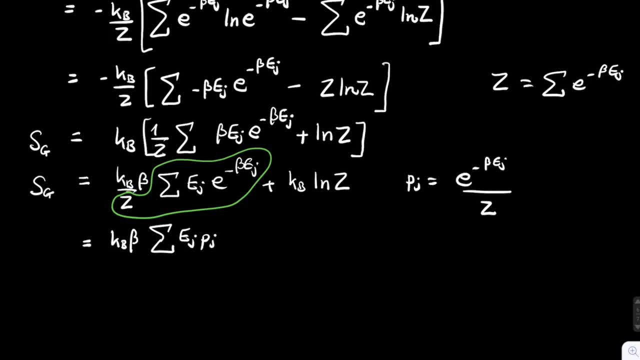 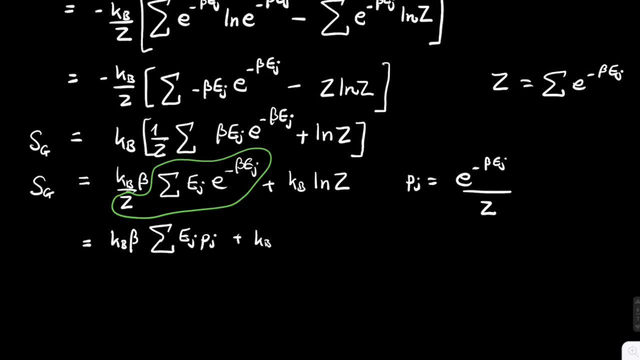 So Pj is simply E to the minus beta Ej divided by Z, plus this Kb, log Z, this final term on the end right here. But what is this? What is sum of Ej, Pj? Well, that is our definition of the average energy U. 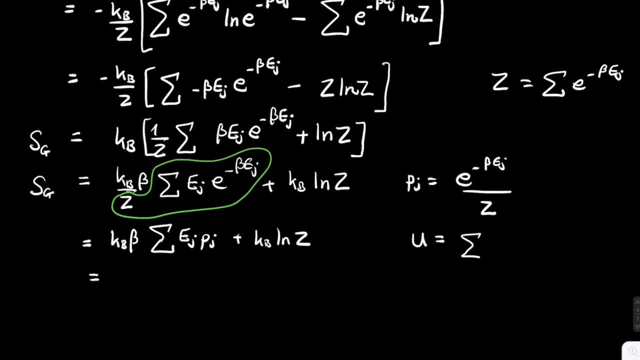 Of course, U is simply the sum, the average if you like, of the probability times each energy. It's our basic statistical thing, right, You know? we take all of them, We multiply the probability multiplied by the energy of that level. 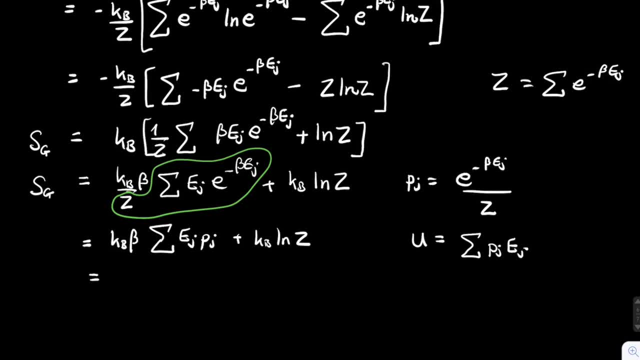 And therefore we end up with the expectation value of our energy. So this term right here, this term is just U, So the entropy is therefore Kb beta multiplied by U plus Kb log Z. Now what are we going to do? 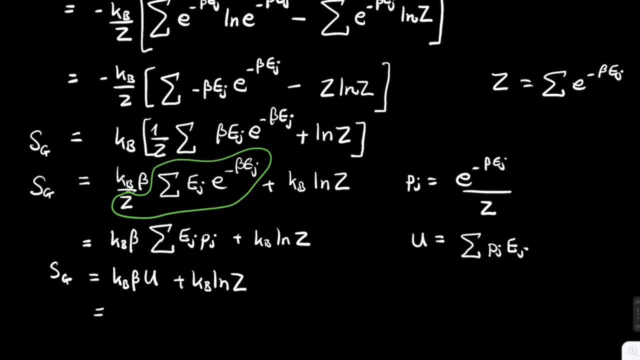 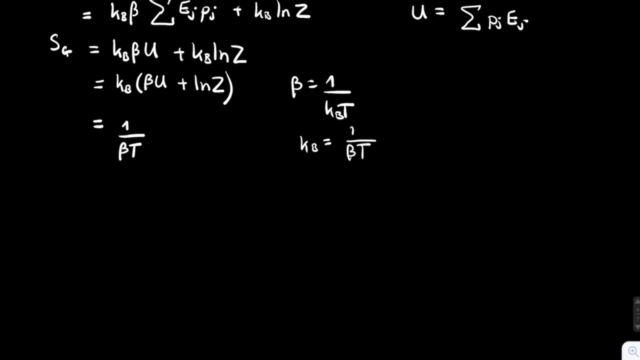 Right around now. Let's just go ahead and sub out Kb. Kb is going to go out the front because it's common on both terms. So the entropy is Kb times beta U, plus the log of Z right here. So I can now write that Kb is simply 1 over beta times T. 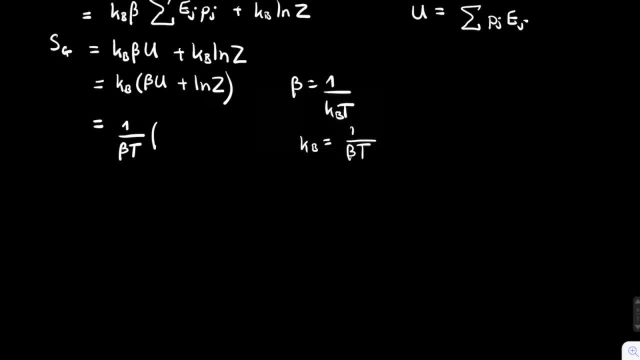 And so therefore, oops, Therefore, we're going to have, And so therefore we can simply write beta U plus the log of Z right there. So let's go ahead and expand out this bracket again, 1.. 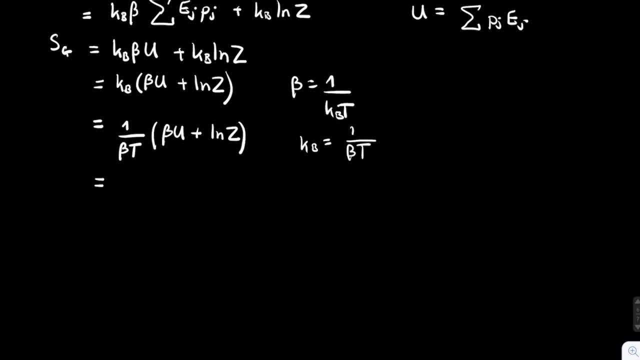 So we're going to get beta U divided by beta T- Well, the betas are going to cancel in the first term, right here. So we're going to get U over T plus log Z divided by beta T. yet again, We can now go ahead and kind of 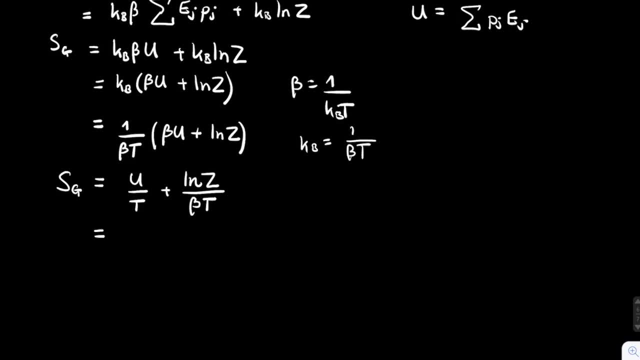 We can multiply this term right here by beta And therefore we can combine the fraction. So SG is simply equal to beta U plus log Z divided by beta T. There we go, So we've got a nice combined fraction right here. 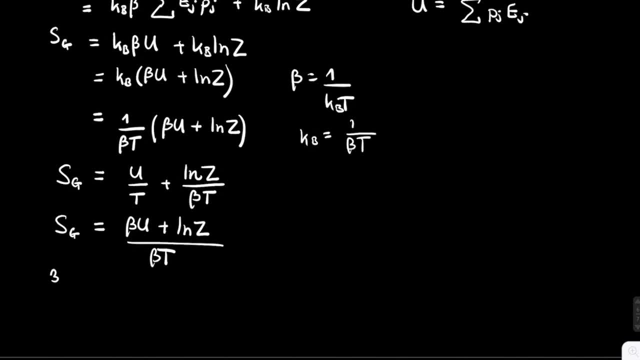 Let's go ahead and get rid of this fraction. So we're going to get beta T times SG is equal to beta U plus The log of Z. And we're going to go ahead and get all the terms with beta. all on one side of the equation. 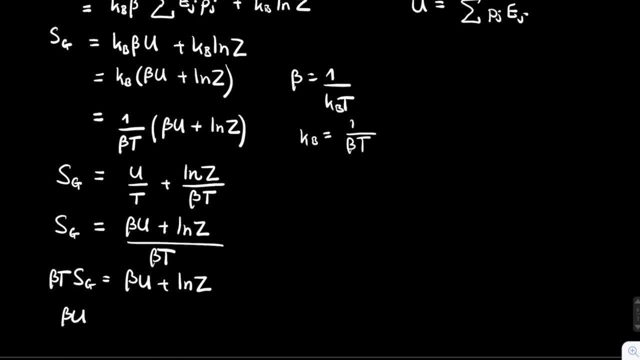 So we're going to have beta U minus beta T SG. So I've subtracted beta SG from both sides. I'm going to get minus the log of Z. Now let's go ahead and divide everything. So I'm going to get U minus beta T SG. 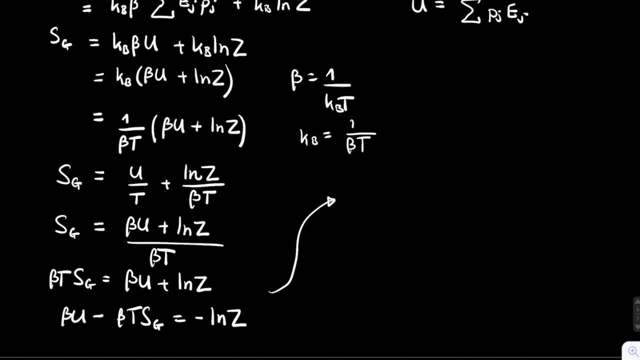 So I'm going to get U minus beta T SG. So I'm going to get U minus beta T SG. So I'm going to get minus 1 over beta. log Z is equal to U minus T S. Hey, this is starting to look pretty cool. 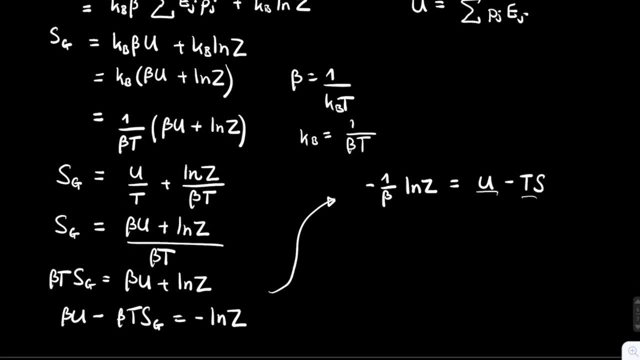 We've actually got mostly thermodynamic quantities. We've got U, T and S. You know this should remind us a little bit of thermodynamics. Hey, we must be getting quite close. Well, if we think back to our video on, 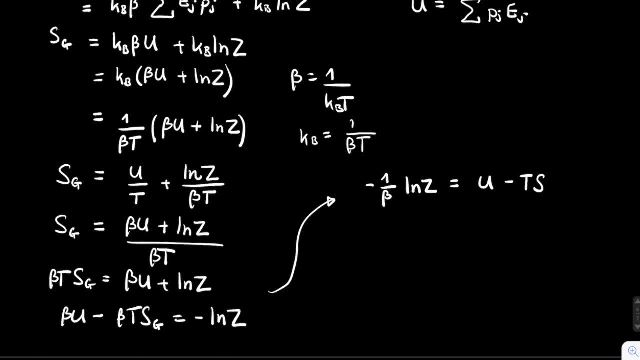 We've got U, T and S. If we think back to our video on thermodynamic potentials, it just so happens that we defined a thermodynamic potential- Remember it was this F term, right here, The Helmholtz free energy. 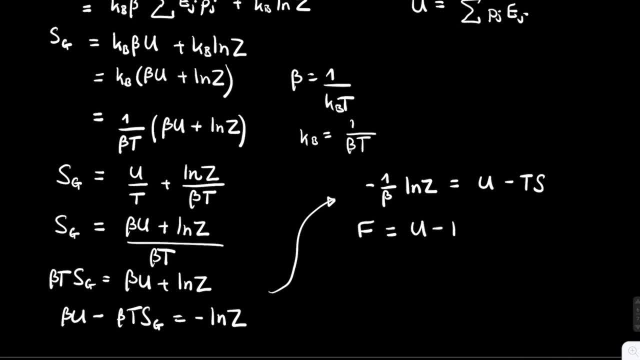 We define this as U minus T S. This is our definition of the Helmholtz free energy. So we've now shown that this F right here is simply equal to minus 1 over beta multiplied by U minus T S. And then we've got this log of Z. 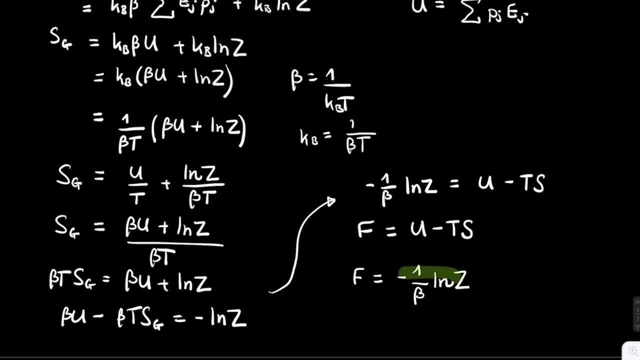 And this is a very important relation. It relates the Helmholtz free energy to this Z right here. But I've not really told you what this Z is, And so we call Z the one particle partition function, And this is a big thing in statistical physics. 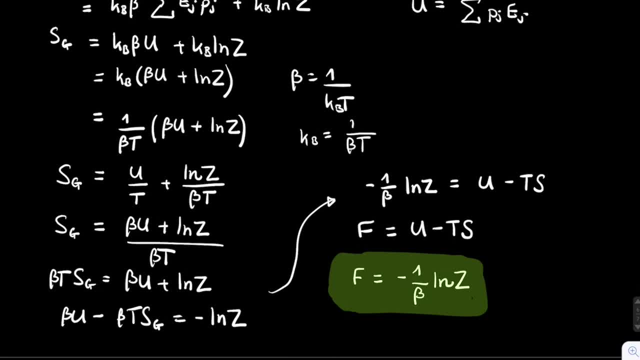 the partition function. We normally give it the symbol Z. This Z in particular is true for one particle, But this relation actually does hold for many particles as well, as we will show in later videos. But just to make sure that we know, it's one particle. 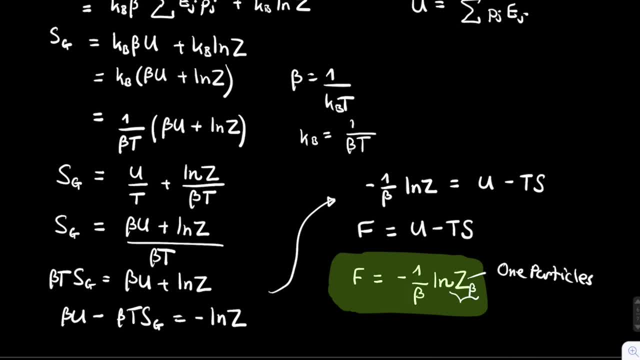 we just simply put a little beta subscript. So this Z beta, which remember we defined as the sum of all the exponentials, is actually called the one particle partition function. And you can see, we can basically immediately get the free energy from this Z.